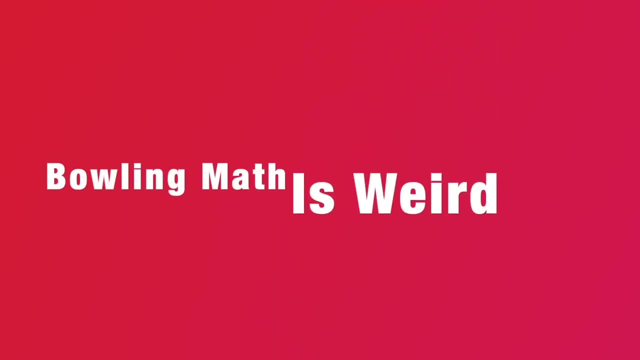 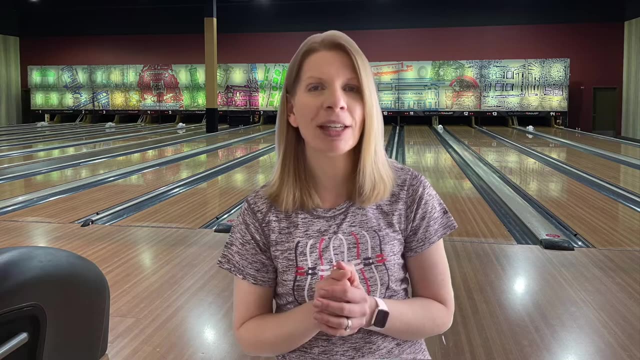 got some tips here today. Okay, bowling math: right, There's 10 frames. So if you get 10 plus 10 plus 10,, 10 times, that should be 100, right? No, bowling math is weird. You would get a 300. 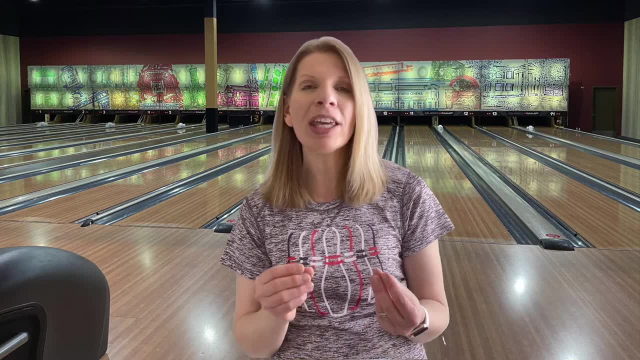 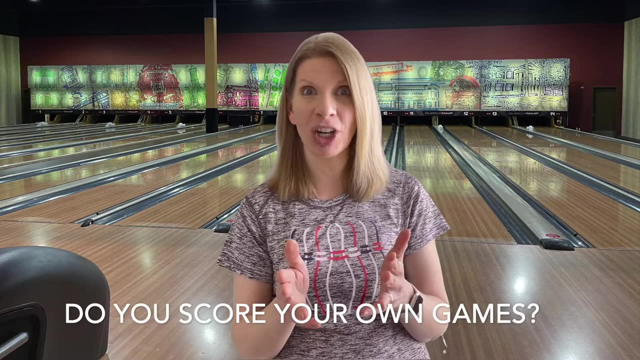 And why is that? I'm going to explain that coming up and why you might want to keep track of your own scores. So I love to keep track of my own scores And I am wondering how many of you ever have kept track of your own scores. 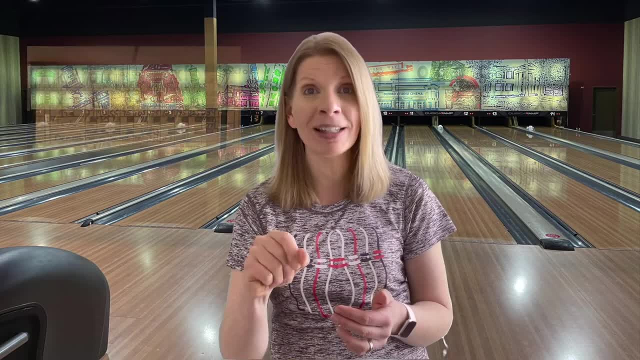 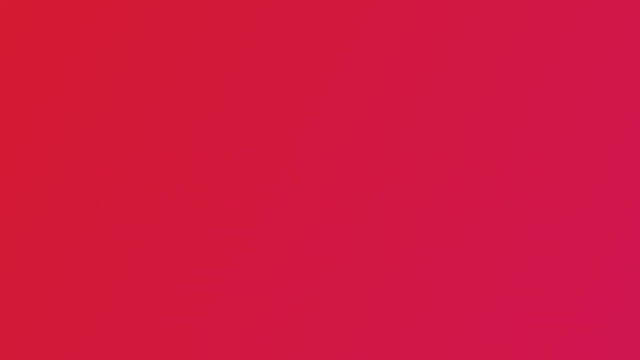 How many of you grew up in the era where we actually had to do pencil to paper, maybe with the overhead projector? Who remembers these days? So when I'm in leagues, I love to keep busy and keeping track and staying focused on what I'm. 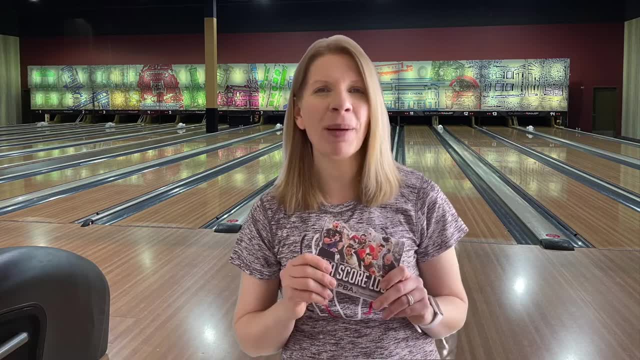 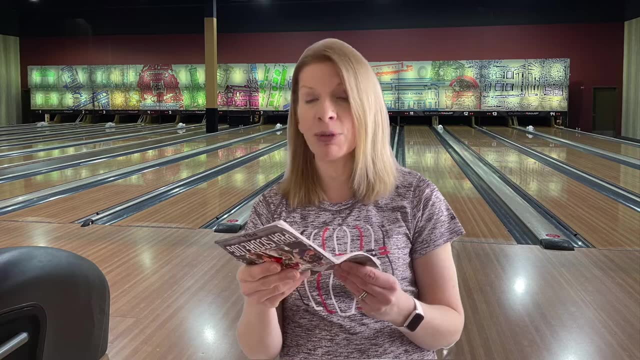 doing on the lanes. So I use this little booklet that my friend brought to me from the Jonesboro PBA tournament not too long ago and I keep track. It has all of the different ways that you can score the pins. You can keep track of what you left, what your score is. You could do the math. 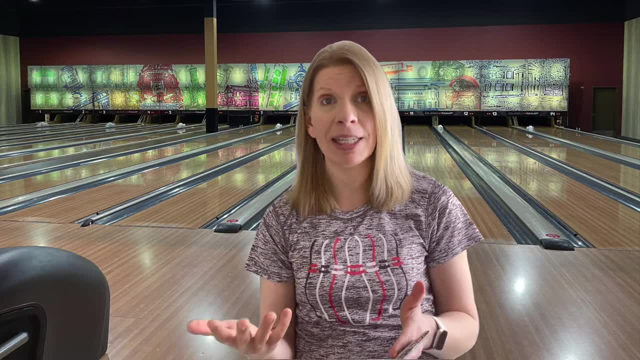 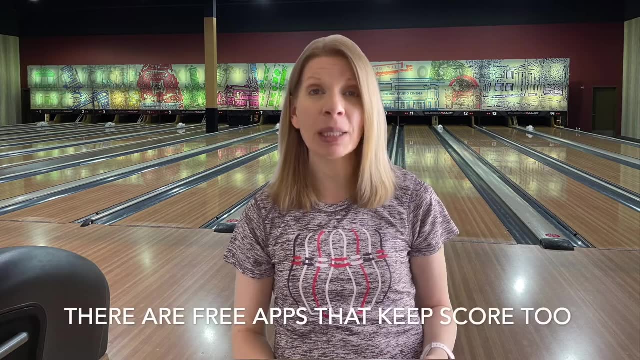 I like to look at it so I can kind of analyze: How many 10 pins did I leave, How many did I make, What percentage did I miss, And I like to keep track of it. that way, You can also purchase booklets online. for these I'll put a link below to some that some of my friends use. 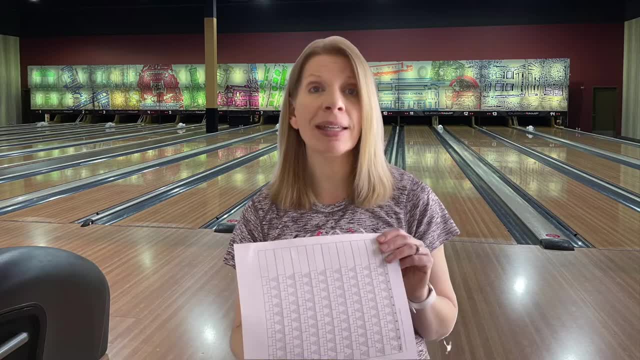 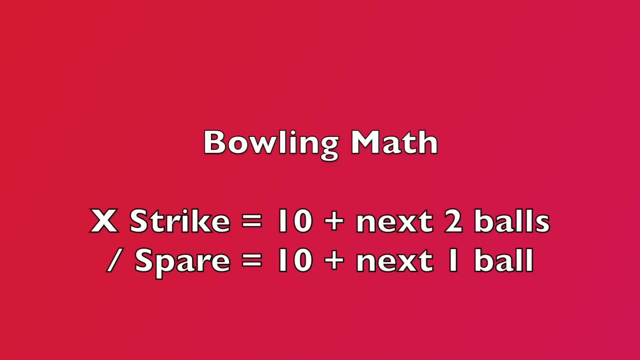 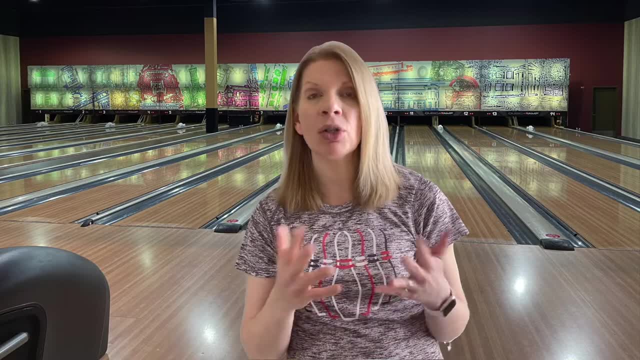 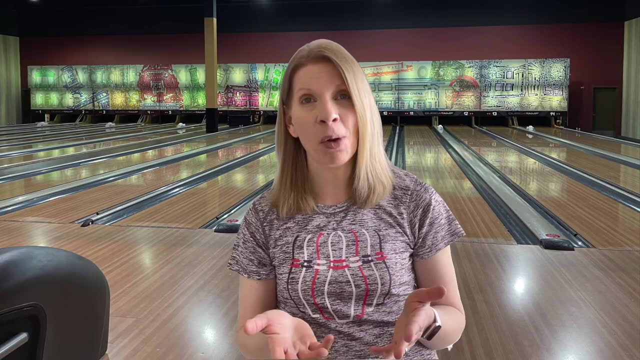 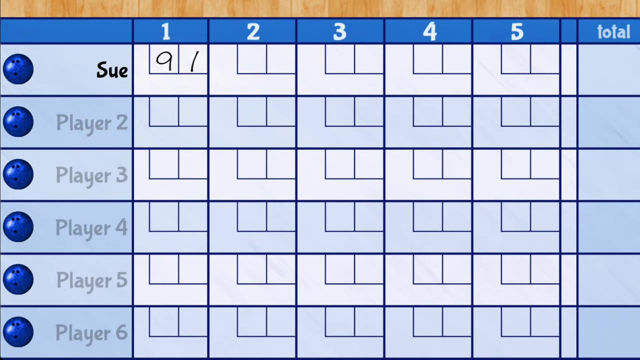 and your second ball. that's a spare, or you can have an open meaning that you don't pick up 10 pins in that frame. Here we have bowler Sue And in Sue's first frame she bowls a nine- nine count and then she picks it up. She gets her 10 pins down with that spare and two balls. 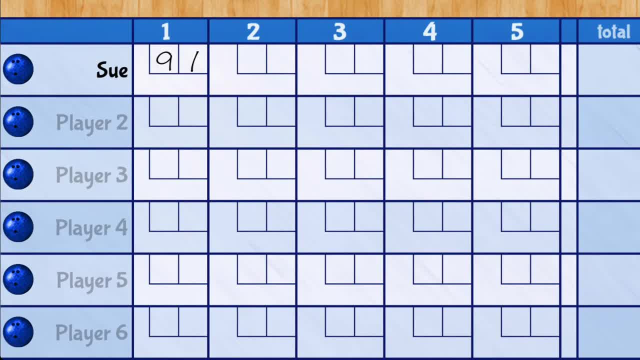 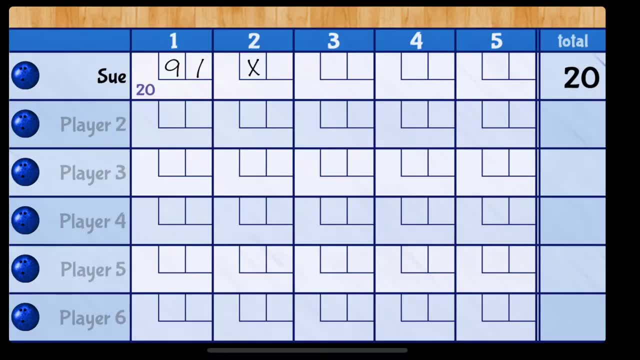 That's considered a spare, And when you score a spare it's 10 plus the next one ball. So we don't know what Sue's score is until she throws the first ball in the next frame. Okay, So frame number two: Sue gets a strike. Good job Sue. So she takes her 10 in that first. 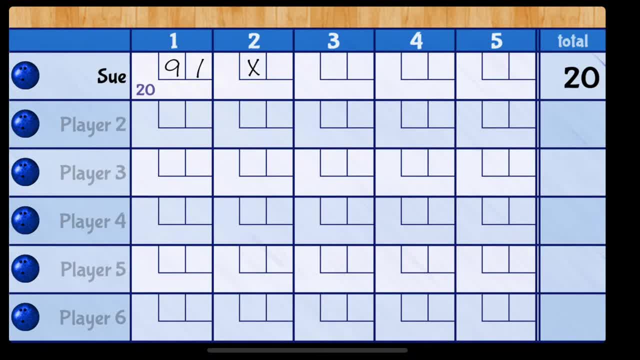 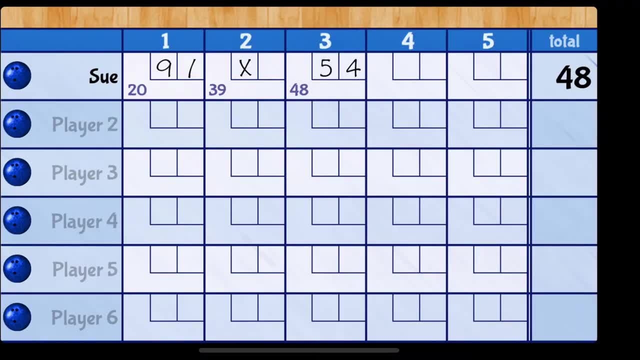 frame plus the next ball, which is a strike equal to 10.. So in her first frame she has a count of 20.. Okay, So frame three for Sue. she throws five, And so she then has to pick that up and she. 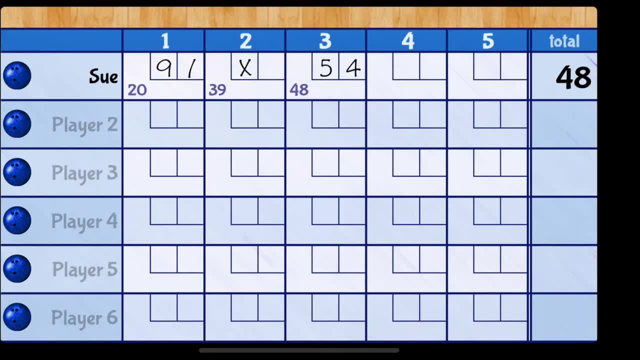 doesn't do it, She gets four down in her next ball. So in frame two we had a strike which is 10 plus the next two balls, And so she's going to add 10 plus five plus four, So 19, to that score. 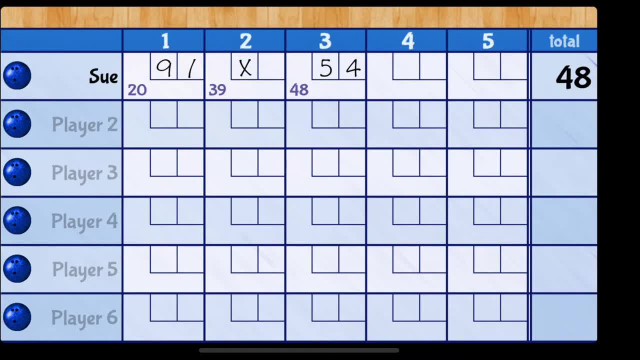 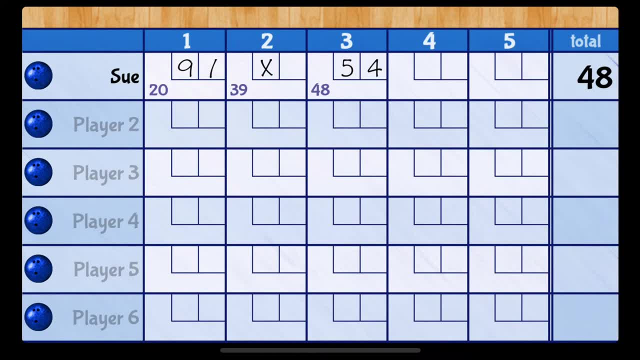 So in frame two she has a score of 39 because she had 20 in frame one. So in frame three, we know we can figure out that score easily, right? Because we add nine pins to what she did in frame two, So she had 39 in frame two. We're going to add nine to that, So 39 plus nine is 48. 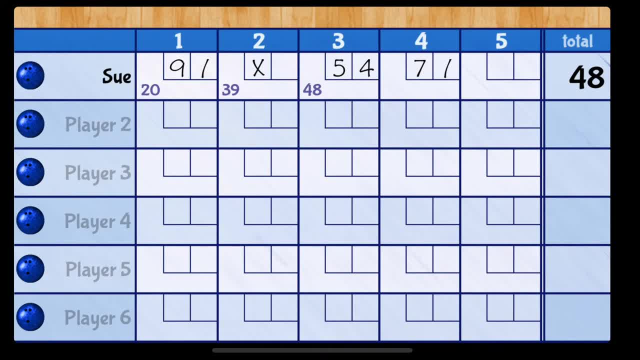 Okay, Frame four: Sue gets seven down in her first count and then she picks up the spare. Good job, Sue. So we don't know what her next score is going to be right, Because we have to wait for the next. 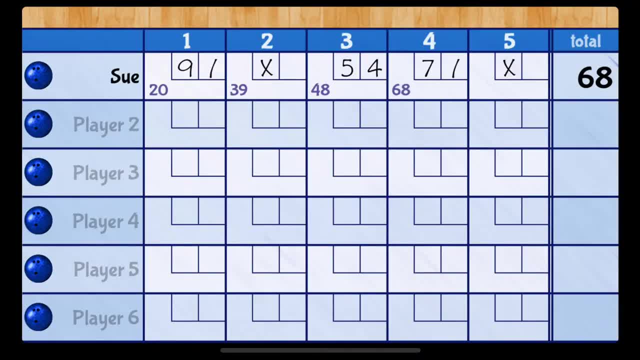 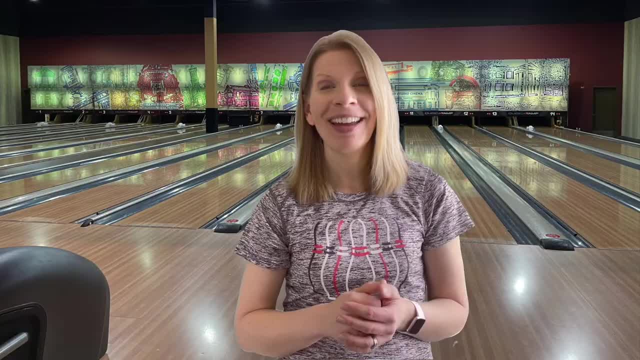 ball. Okay. So frame five: Sue scores a strike, So we are adding 10 to that spare that we shot in frame four and that makes that 68 in frame four. Now for frame five. we have to wait for the next two balls to see what Sue's score is going to be. 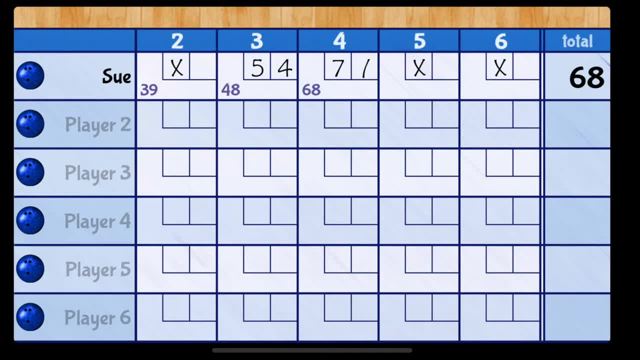 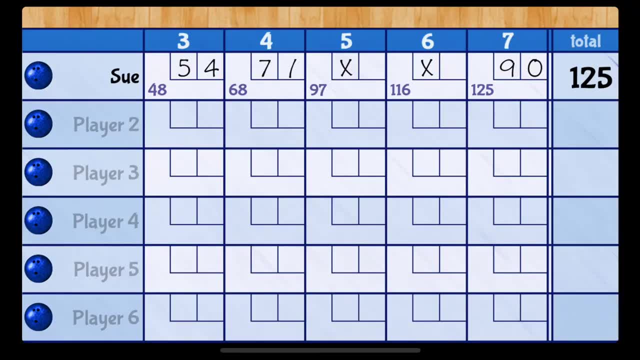 Okay. So frame six: she throws another strike. We're still waiting to score this because the strike is 10 plus the next two balls. Okay, So frame seven: Sue gets a nine count in her first ball. So we can go backwards and we can start scoring some of this. So we can go back to frame. 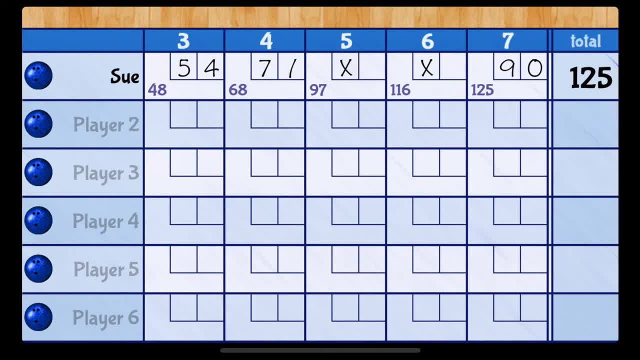 five She had a strike plus the strike in frame six plus the nine, and that gives her a 97 count in frame five. Now in frame six, we're still waiting. She doesn't pick up her spare in frame seven, So we're adding 10 plus the next two balls, which is total of nine, So 19.. So in frame 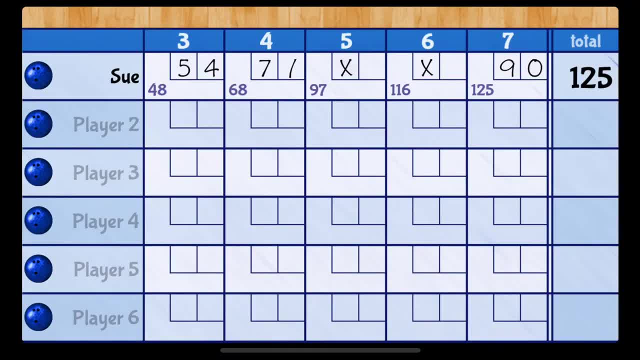 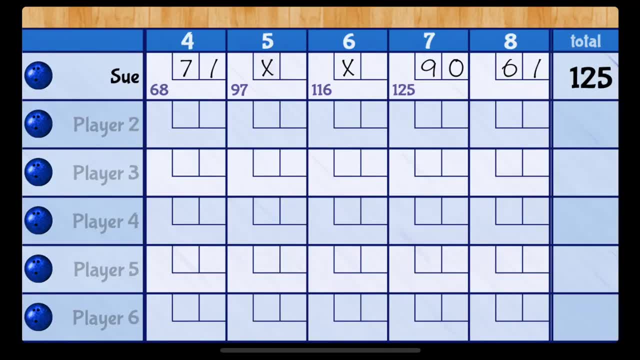 six she has 116. And we know in frame seven she has no strikes and spare. So we're just adding nine, making that 125.. So in frame eight she has a six count and she picks up her spare. So we're waiting. 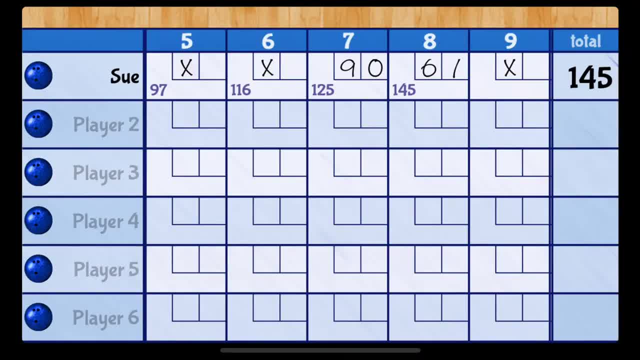 on the next ball, in frame nine, to see what the score is. And in frame nine she throws a strike. So we're adding another 10 pins to that. So 10 plus 10, that's another 20 to her score. See how the math compounds. So in frame eight,